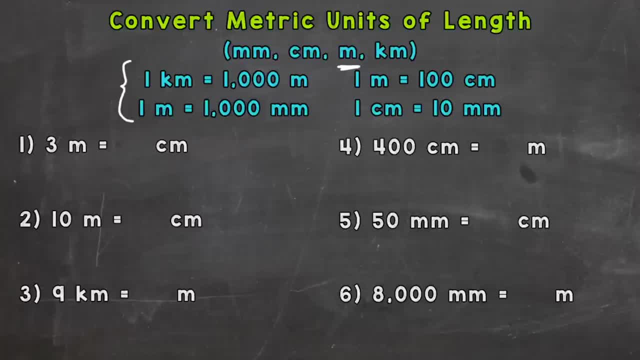 but how wide. a staple is, And on most rulers centimeters will be marked on the metric portion of that ruler. And then a meter is a little over a yard, So a meter stick a little longer than a yard. And then kilometer is a little over a half mile, So kilometers are used to measure long. 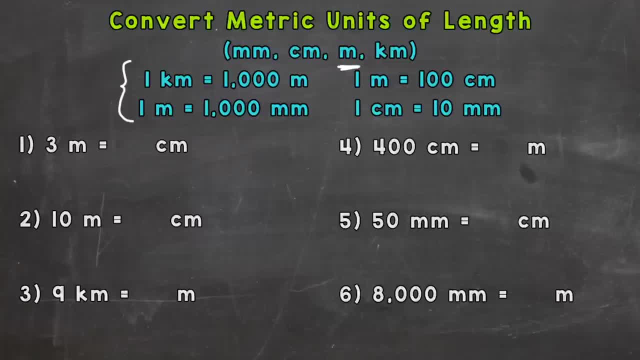 distances. So let's get into some conversions here. And number one: we have three: meters equals how many centimeters? Well, one meter is a hundred centimeters. So we have three. One hundred one hundred one hundred. And whenever we go to meters, to centimeters, we multiply by a hundred. So three meters equals three. 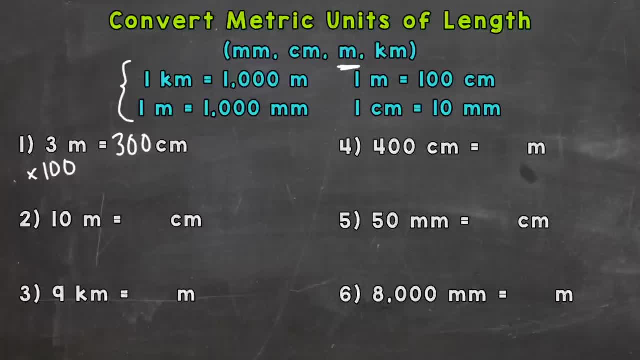 hundred centimeters. Next we have ten meters equals how many centimeters? So again, meters to centimeters. multiply by a hundred. Each one of those meters is a hundred centimeters and we have ten of them. So let's multiply and we get ten times a hundred. 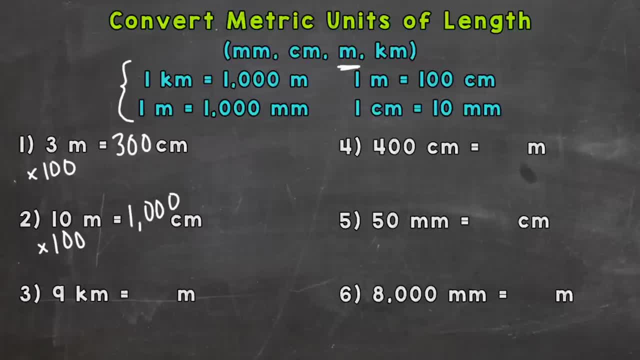 equals a thousand centimeters. Number three: nine kilometers, equals how many meters? Well, in one kilometer we have a hundred centimeters. One kilometer, there's one thousand meters and we have nine of them. So a thousand, a thousand, a thousand nine times, or nine times a thousand. 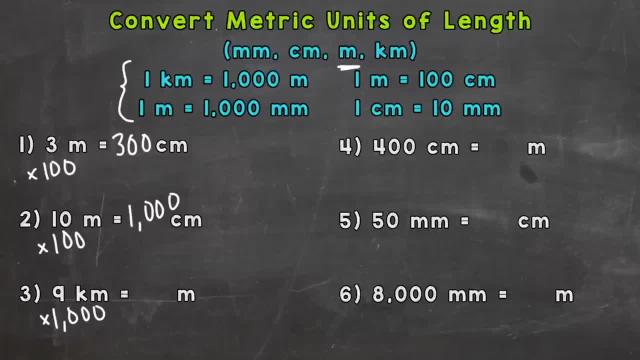 So when we go kilometer to meter, we multiply by a thousand, And for this one specifically we get nine thousand. Number four, four hundred centimeters equals how many meters. Number four, four hundred centimeters equals how many meters. Well, each meter there's a hundred centimeters. So we need to take that four hundred and split it into groups of one hundred. 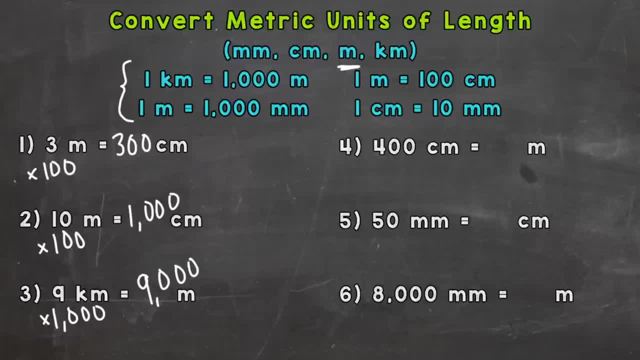 Each one of those groups of one hundred equals a meter. So we need to do four hundred, divide it into groups of a hundred or meters there, And we end up with four. So centimeter to meter, divide by a hundred Number. five millimeters to centimeters, equals how many meters? 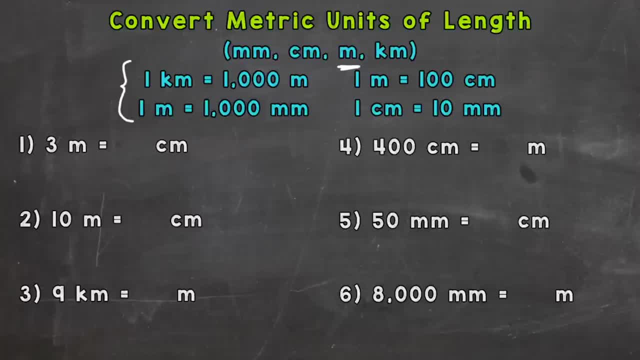 of length. So it's a very small unit of length. So it's a very small unit of length And on most rulers centimeters will be marked on the metric portion of that ruler. And then a meter is a little over a yard, So a meter stick a little longer than a yard, And then kilometer is a. 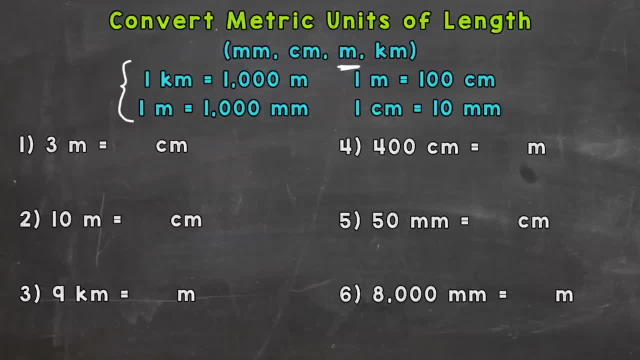 little over a half mile. So kilometers are used to measure long distances. So let's get into some conversions here. And number one: we have three meters equals how many centimeters? Well, one meter is a hundred centimeters. So we have three: One hundred one hundred one hundred. 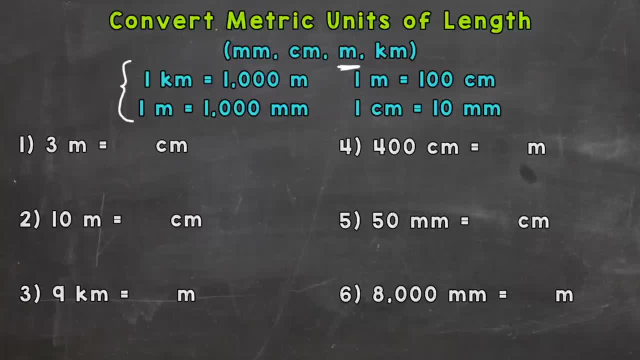 And whenever we go to meters to centimeters, we multiply by a hundred. So three meters equals three hundred centimeters. Next we have ten meters, equals how many centimeters? So again, meters to centimeters, multiplied by a hundred. Each one of those meters is a hundred. 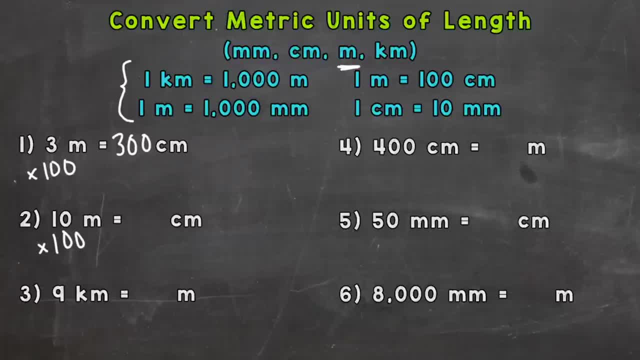 centimeters, and we have ten of them. So let's multiply and we get: ten times a hundred equals a thousand centimeters. Number three, nine kilometers, equals how many meters? Well, in one kilometer there's one thousand meters and we have nine of them, So a thousand, a thousand a. 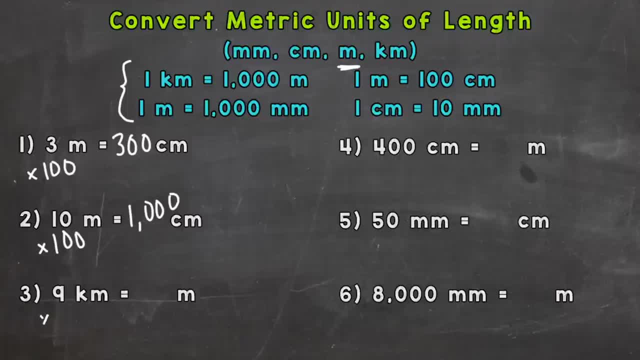 thousand nine times or nine times a thousand. So when we go kilometer to meter, we multiply by a thousand And for this one specifically we get nine thousand. Number four, four hundred centimeters equals how many meters? Well, each meter there's a hundred centimeters, So we need to take that four. 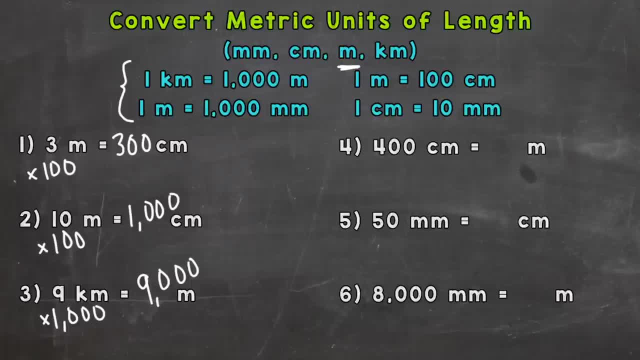 hundred and split it into groups of one hundred. Each one of those groups of one hundred equals a meter. So we need to do four hundred, divide it into groups of a hundred or meters there, and we end up with four. So centimeter to meter divide. 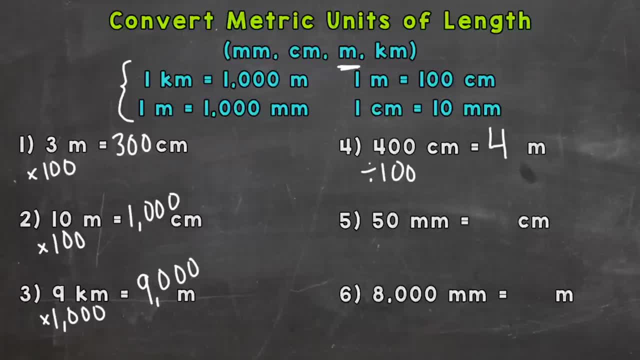 by a hundred Number five millimeters to centimeters. So there are ten millimeters in every centimeter. So we need to divide by ten or split into groups of ten. Each one of those tens is a centimeter. So fifty divided by ten gives us five centimeters. So millimeters to centimeters divide by. 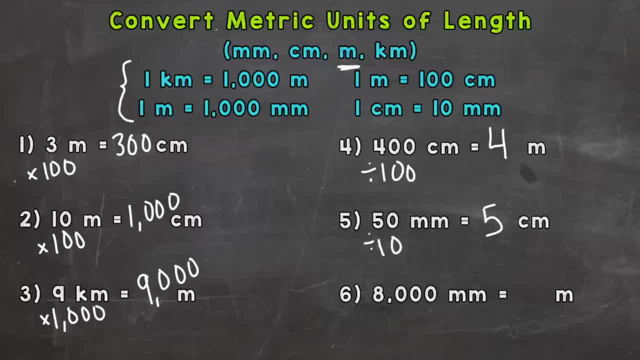 ten Number six. eight thousand millimeters equals how many meters? Well, there's a thousand millimeters in every meter. So we need to split that eight thousand into groups of a thousand. Each one of those thousands is one meter. So millimeters to meters divide by a. 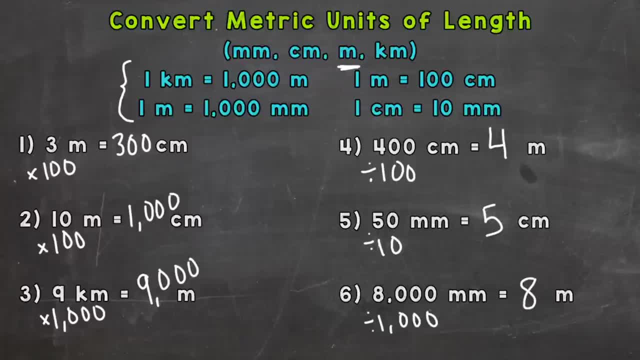 thousand and we get eight meters. All right, so there's there, you have it. There are some basic conversions within metric units of length, Specifically millimeters, centimeters, meters and kilometers. Thanks so much for watching. Until next time, peace. 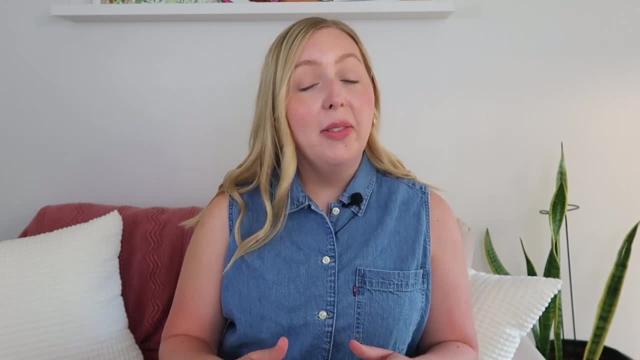 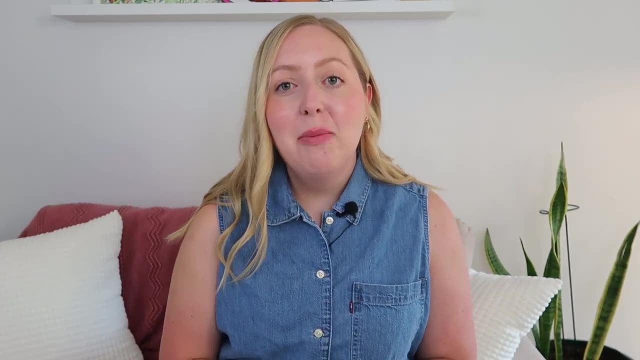 So it's the first day of music and you have your fourth, fifth or sixth grade students ready to go. What do you teach them? Let's talk about it. Hi, if you are new to my channel, my name is Jessie. I am a kindergarten through sixth grade music teacher here in Arizona and on this channel. 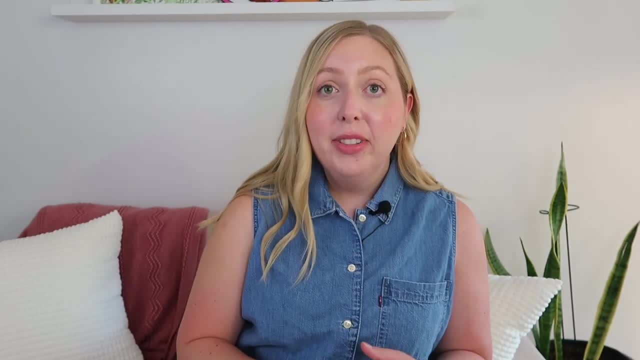 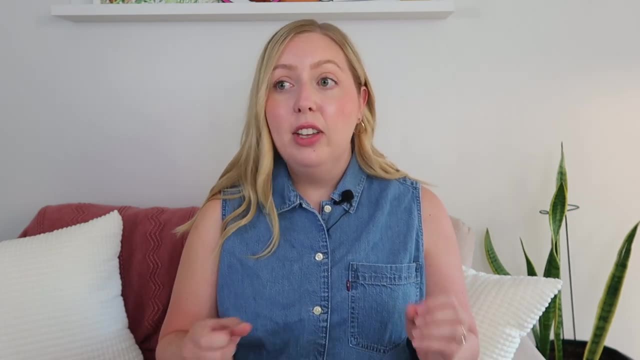 I talk about organization and planning. I talk about modern lesson ideas and also ukulele, All right. I don't know about you guys, but the first few lessons are always tricky. Every year I feel like I'm kind of like: what do I want to do? What do I want to teach? And honestly, I do. 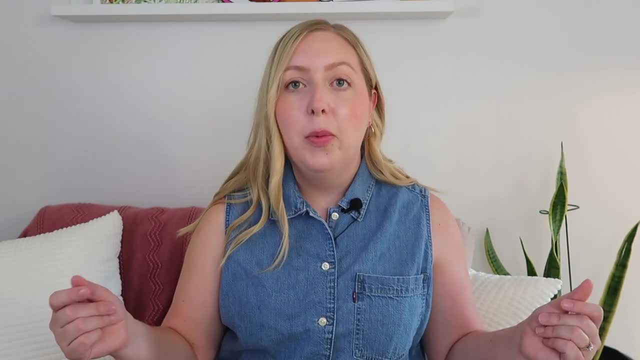 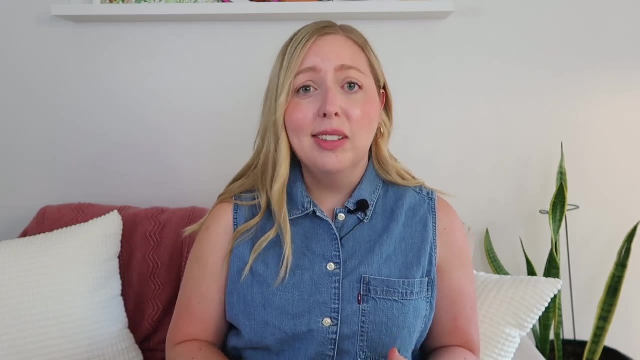 want to say, and every year I like want to jump into something fun and right away- and there are some you know, we can do that, We can do that and we'll get to that. But also the first day, second day, it's kind of really seating chart and lesson rules, right And procedures. I think that 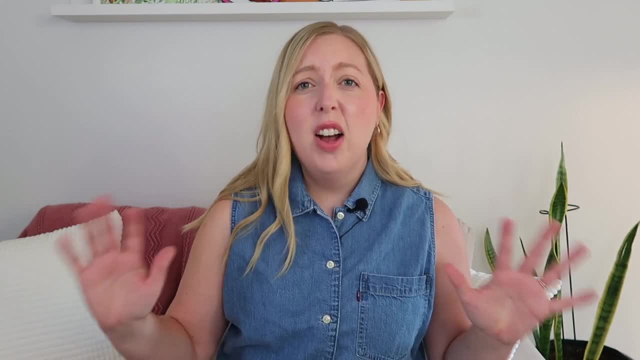 you know, sometimes I put so much pressure on myself that music has to be this just fun thing all the time. But honestly, if we all get on the right page, we're all you know. we know we're going to get there, We're going to get there, We're going to get there, We're going.